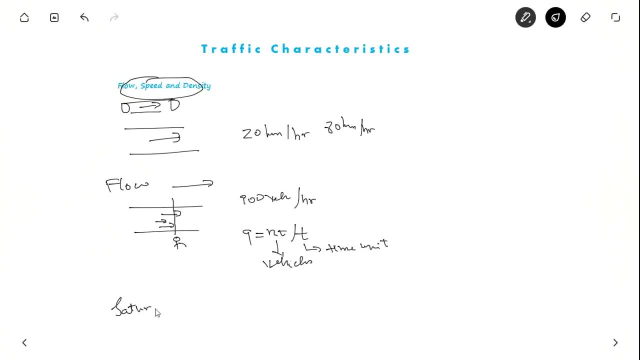 varies. Yes, Saturday there will be a different pattern, because people don't go to offices Saturday and Sunday, And in monsoon season it will be different. So we have different types of measurement. So we will see the different types of traffic flow measurement. 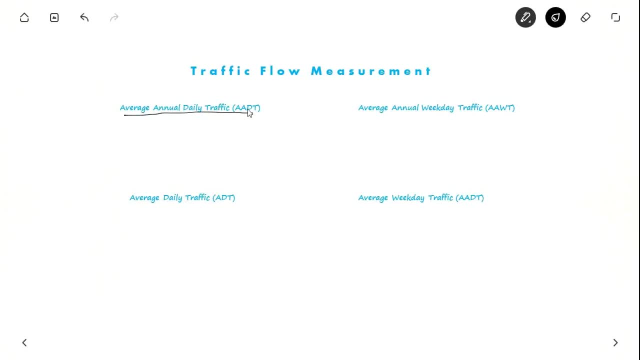 First we will see about annual average daily traffic. It is nothing but traffic flow over averaged over all the 365 days. Suppose you observe n vehicles in a year, n divided by 365 is annual average daily traffic, And average annual weekday traffic is nothing but which is observed only for the weekday. 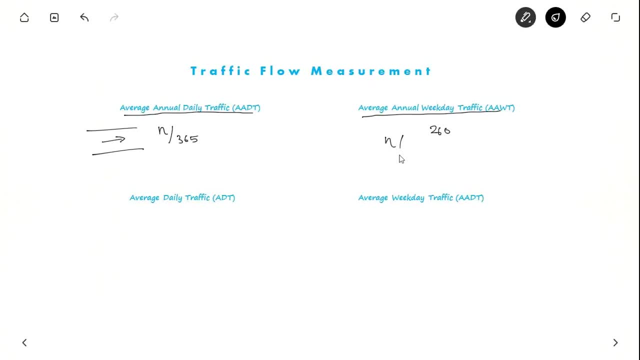 Suppose there are two 60. Weekdays in a year, N vehicles divided by 260 days, that is average annual weekday traffic, Average daily traffic. it is nothing but n divided by ustha is observed. Suppose you are in a company. you cannot obviously measure the traffic for all the 365 days. 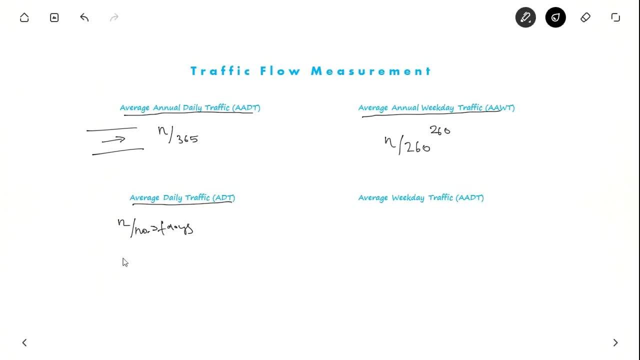 So you will measure the traffic, say, for eight days. So if n vehicles passed in a year days, N divided by 8 is the average daily traffic, and if the same thing you do only for weekdays, it is average weekday traffic. Whatever we saw, 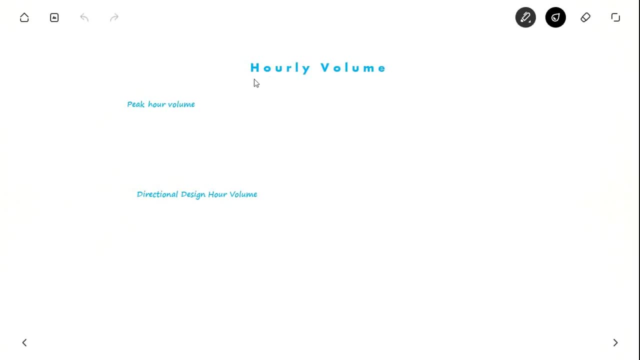 now was per day traffic. We also have hourly volume. Often you observe that in the morning there is a high volume because people go to offices, say from 9 to 10. During 9 to 10 you observe very high volume. that is the peak R volume. So 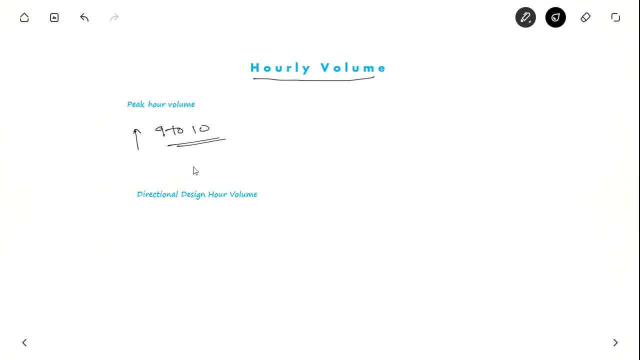 this is used for traffic facility design, etc. Directional design, R volume. So this is derived from the AADT. It is nothing but AADT into K, into D. K is nothing but the proportion of traffic in the P car. Suppose 9 to 10, you observe 100 vehicles and for the 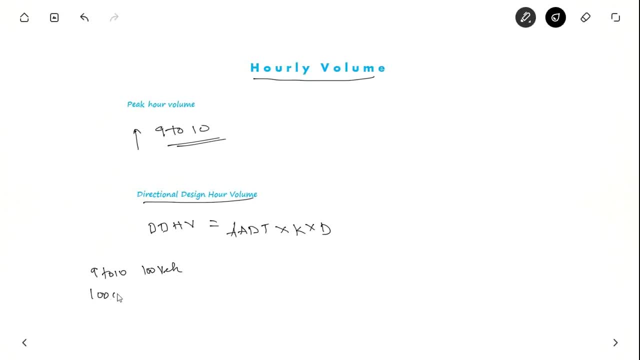 whole day you have observed 1000 vehicles. So K is nothing but 100 by 1000. that is 0.1 and D is the directional flow. Suppose you have observed 1000 vehicles in a day and this side 700 vehicles passed and this side only 300 passed. So directional factor is 700 by. 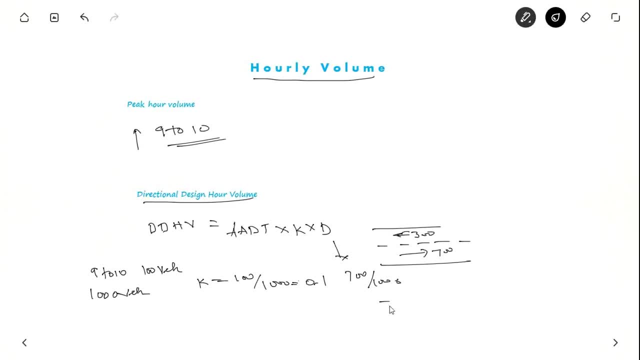 1000, which is 0.7.. So directional designer volume is average annual daily traffic into K, into D. So this is the directional flow. Often we see that K is taken from the 30th highest P car volume. 30th highest P car volume. 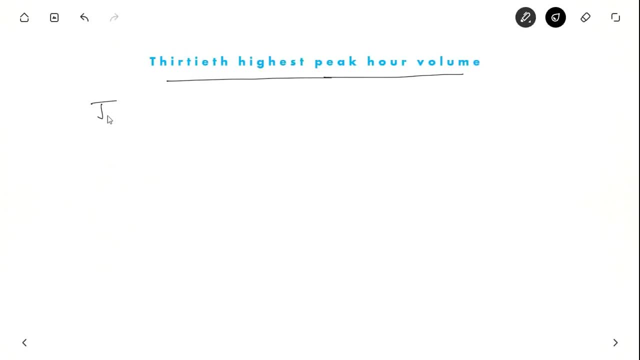 is nothing. but suppose, say, in a year you take Harley traffic, Suppose, on July 9th, 9 to 10, you observed 1000 vehicles per hour. that is the highest volume in an hour observed over the year, And similarly on June 10th. 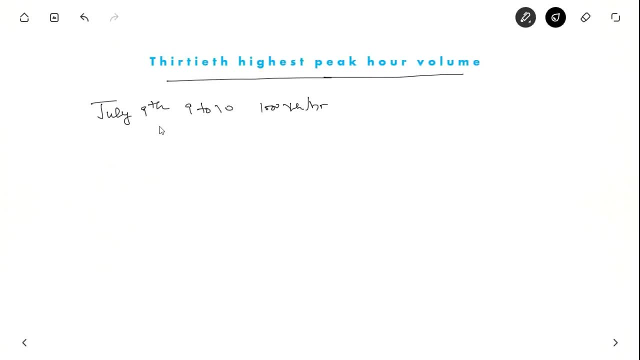 you observe 900 vehicles per hour. Similarly, if you go on, you find the 30th highest peak R. So that is the 30th highest peak R volume That is used in the calculation. So directional designer volume equal to 30th peak R volume into directional factor. We will see what. 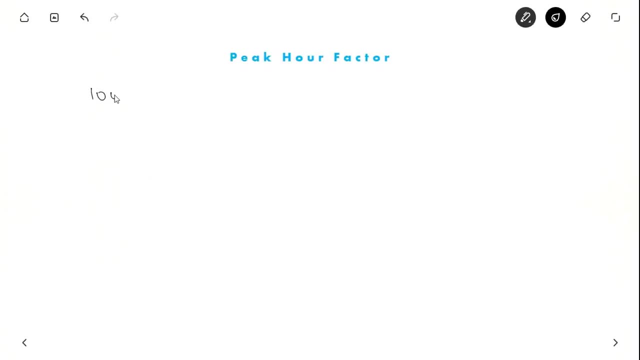 is peak R factor. Suppose say, 1000 vehicles pass in 15 minutes, Then the flow is 4000 vehicles per hour, 1000x4.. Because in 1 hour there are 60 minutes, 60 divided by. 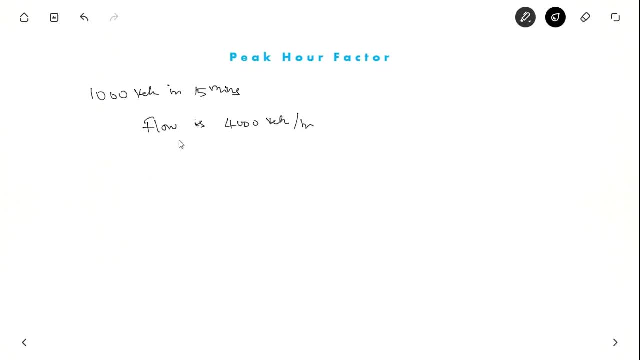 15 is 4 and 4x1000 is 4000.. Say, 5 to 5.15pm the flow is 1000 vehicles And 5.15 to 5.30, the flow is 800.. And 5.30 to 5.45, the flow is 600.. 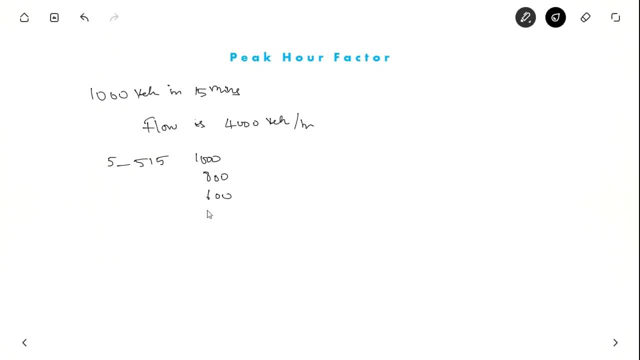 600 and 545 to 6, the flow is 600. so total flow from 5 to 6 is 3000 vehicles per hour. the relation between this 3000 and 4000 is peak R factor. peak R factor is nothing but hourly volume divided by maximum rate of flow. so for this 15 minutes, peak R factor equal. 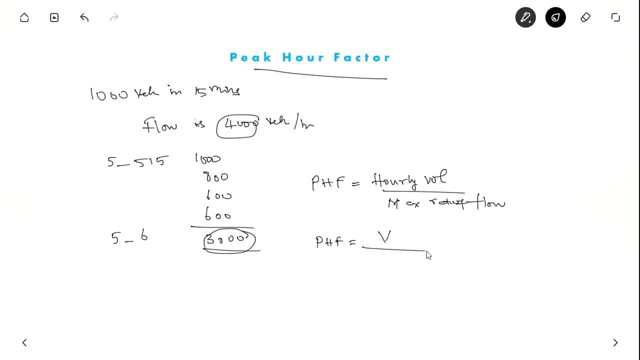 to hourly volume V divided by 60, divided by 15, that is 4 into the volume rate of flow in that 15 minutes. so it is equal to 3000 divided by 4 into 1000, which is nothing but 0.75. this is peak R factor. 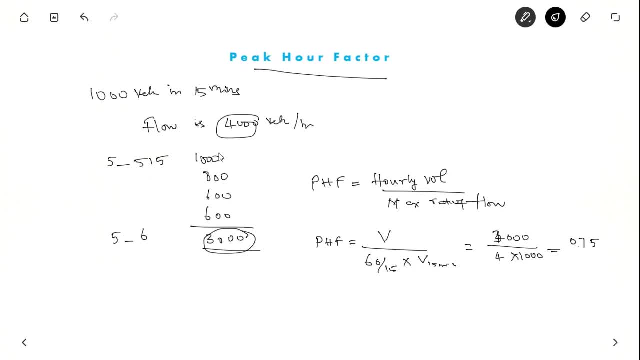 why do we use peak R factor? because in 15 minutes sometimes very high volume will come which the road cannot handle. so that is why we use peak R factor in design. the second most important traffic parameter is speed. first let us see what is sport speed. suppose you stand at a point and you observe the instantaneous speed of the vehicle, like when you see a speedometer. 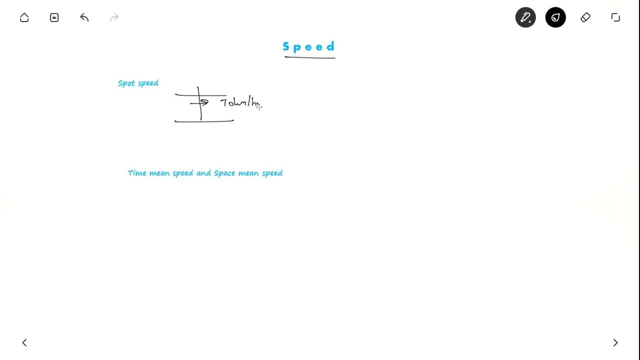 it is transferable after any vehicle. you can see that the degrees are responsible, especially in the wind speed. also there is the speed. each speed methods has an impact on the delivery of traffic hours. time speed, in this particular Hinreich per can Van blev a point that is of binary energy. that could be 70 kilometer per hour, 80 kilometer per hour for any vehicle. so that is the sport speed. there are two important measures of speed with their time means, speed app space mean speed. let us see what is timing speed: time in speed we will denote by the T, and space means we will denote. 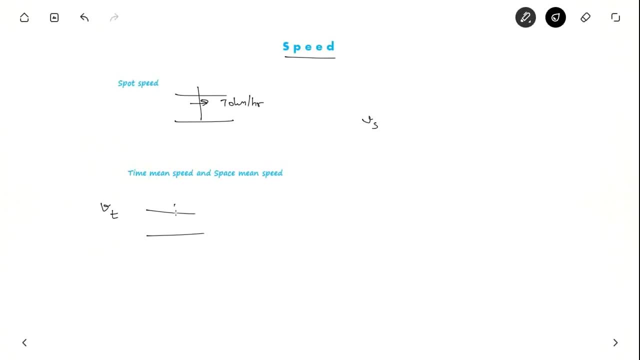 the V T and space means speed, will denote V S. suppose you are standing at a point and we are standing at R, factor for 2 seconds for it to be V T, then M is not a Huhh point and you observe the speed of vehicles crossing this point over a. 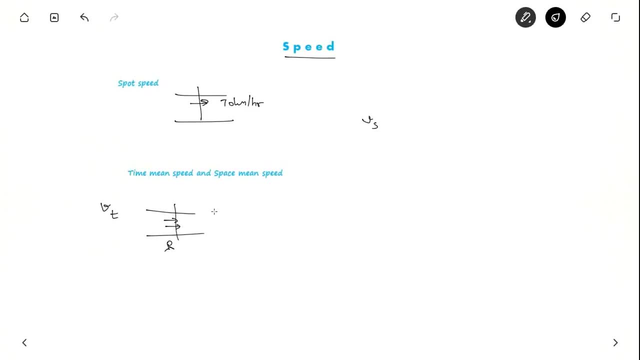 specific period of time. Suppose you have observed, say, three vehicles of speed: 50,, 60 and 70. The instantaneous speeds are 50, 60 and 70 kilometer per hour. So the time in speed is nothing but 50 plus 60. 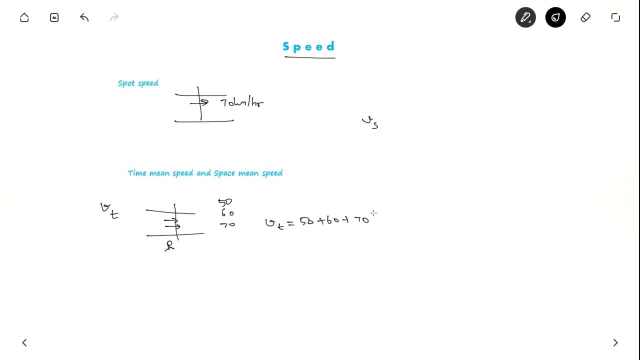 plus 70 divided by 3, which is 60 kilometer per hour. So time in speed is nothing but summation of the vehicle speeds divided by number of vehicles. Let us see what is space mean speed? Space mean speed is nothing but the average of. 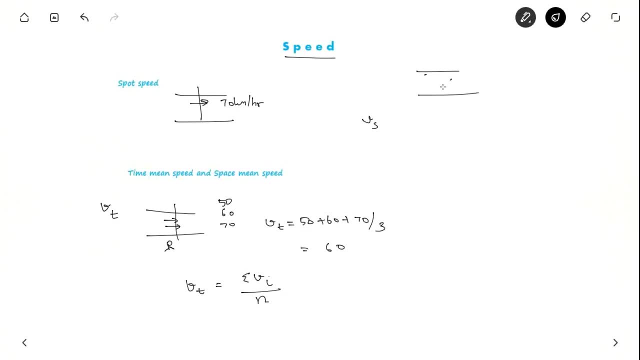 all the speed of the vehicles over a section. Suppose say we define a one kilometer section. So there are different vehicles with different speeds. If you average them, that is the space mean speed. Suppose say it takes Ti time for each vehicle to cross this one kilometer. 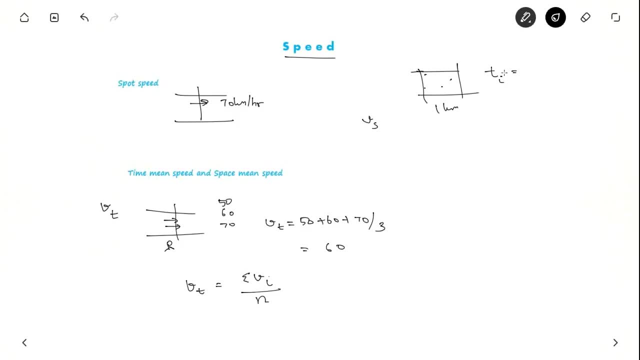 They are going at, say speed of Vi So Ti is equal to 1 by Vi, So the average time taken for all these four vehicles will be sigma Ti by N, So equal to 1 by N into Sigma 1 by Vi So T average for this one. 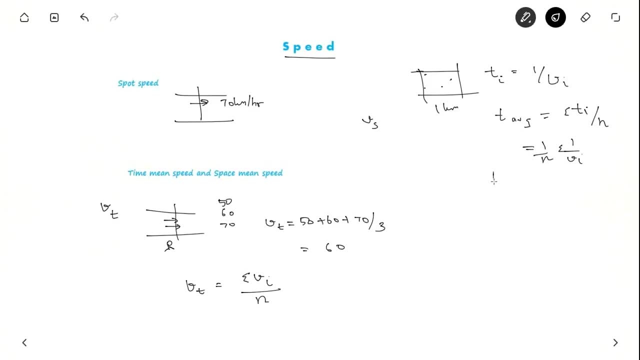 kilometer is nothing but 1 by Vs. So 1 by Vs equal to 1 by N into Sigma 1 by Vi. Vs is equal to N divided by Sigma 1 by VI. So this is the harmonic mean of different speeds. So if 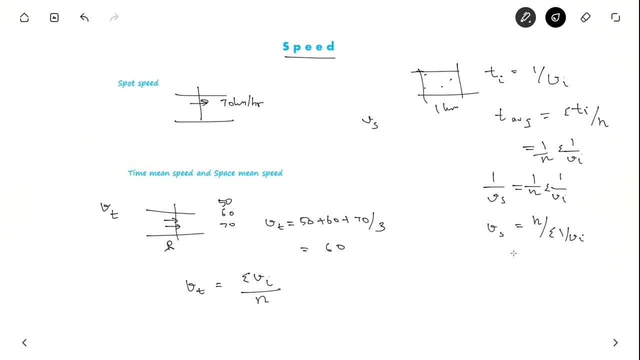 the speed of the vehicles were 50, 60 and 70. So Vs equal to 3 divided by 1 by 50 plus 1 by 60 plus 1 by 70. This will come around 59, 58 point something. So this is space. 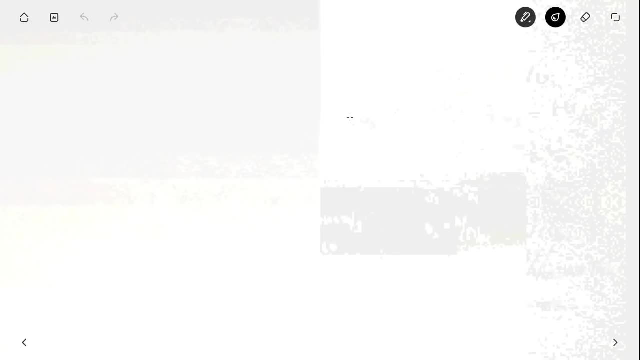 mean speed. Another interesting fact is that the space mean speed is always less than the time mean speed. This is because the slower moving vehicle is given more weightage in space mean speed, That is, they occupy the road stretch for a longer amount of time. Let us solve a problem. 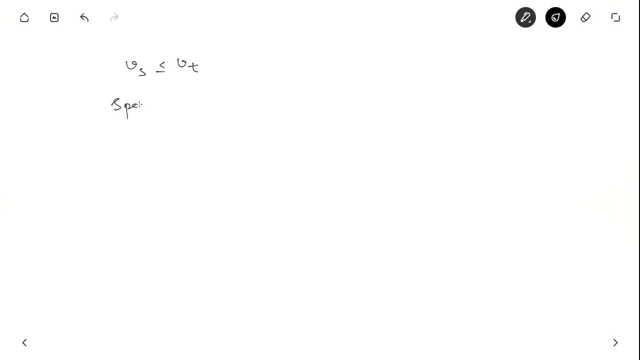 and see Different speed ranges are given. So 45 to 55 kilometer per hour, there is one vehicle. 55 to 65 kilometer per hour, there are two vehicles. 65 to 75 kilometer per hour, again there is one vehicle. 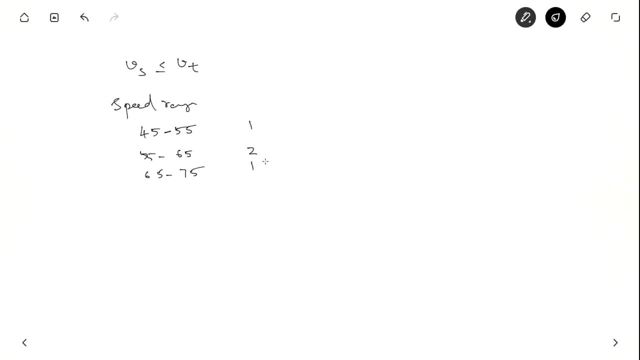 Again, there is one vehicle, So let us find out the space mean speed and time mean speed. So 45 to 55, the average speed is 45 plus 55 divided by 2, which is 50, and it is 60 and this is 70.. 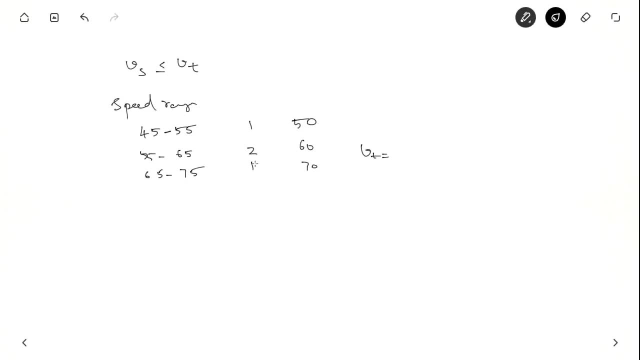 So time mean speed is the arithmetic mean of all this. So it is one into 50 plus two into sixty plus 16 Graph. Where is my average speed? It is 45 plus 55. divided by 2 it is 50, and this is 60 and this is 70.. So time mean speed is the arithmetic mean of all. 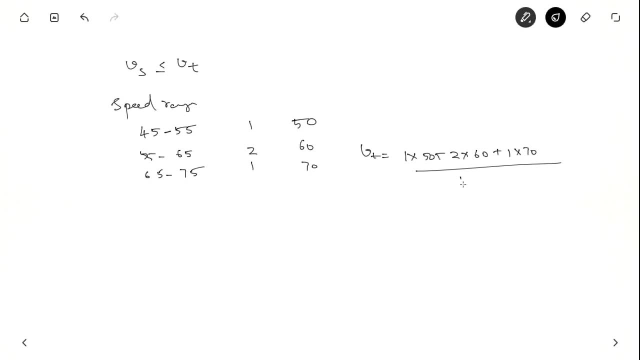 as 1 into 70, divided by 1 plus 2 plus 1,, which is equal to 4,. 120, 190, 240,, 240 by 4,, which is 60.. 60 km per hour is the time mean speed. Let us see what is the space mean speed It. 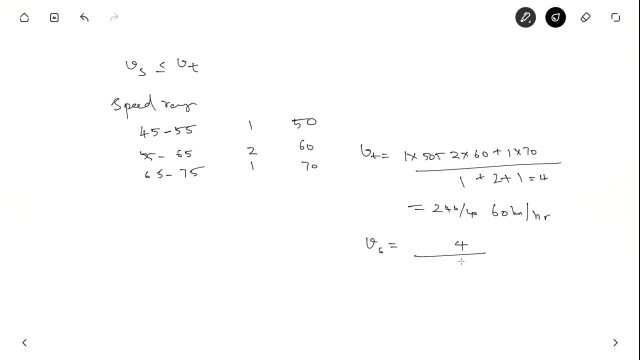 is nothing but 1 plus 2 plus 1, that is 4, divided by 1 by 50 plus 2, into 1 by 60 plus 1 by 70. This is equal to 59.15.. As you see, 59.15 is less than 60 km per hour.